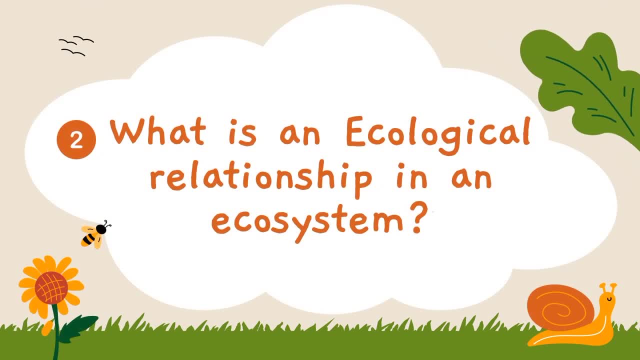 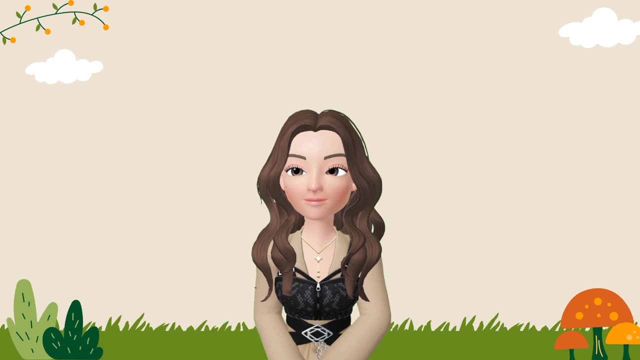 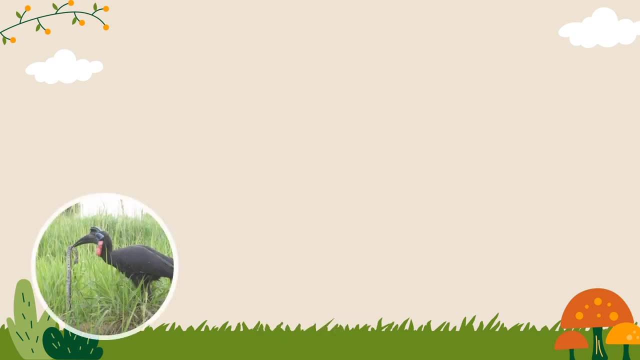 Now, what is an ecological relationship? in an ecosystem, All organisms are connected to each other. in an ecosystem, Organisms form relationship with each other because they are connected. Some organisms compete against each other for resources or space, while other organisms depend on each other for survival. 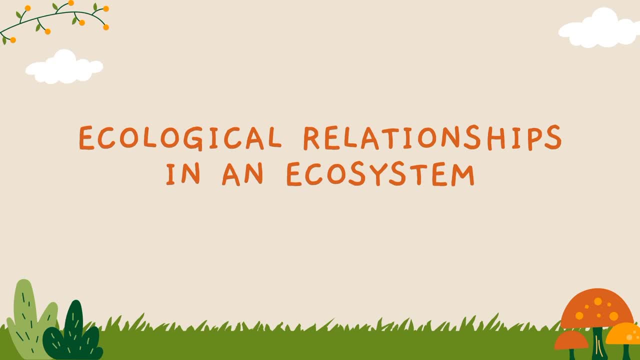 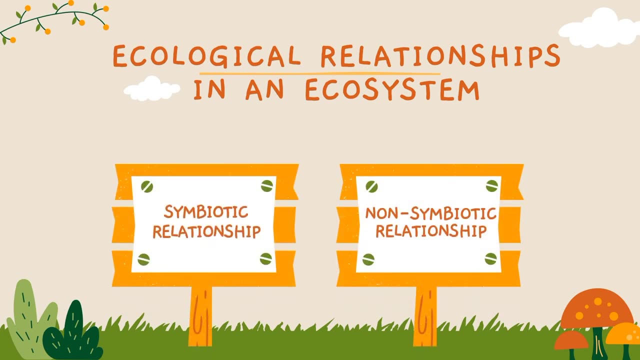 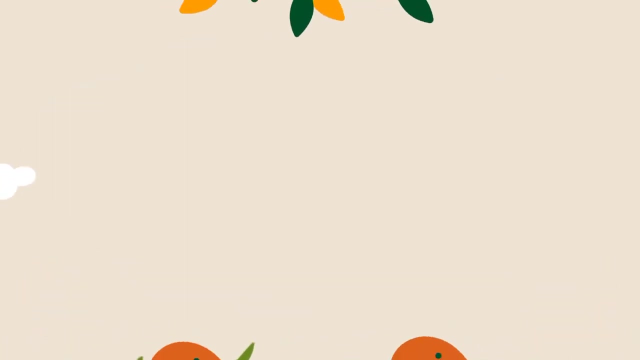 Now these relationships are called ecological relationship. Ecological relationship can be symbiotic or non-symbiotic. Now what do you think is the difference between symbiotic and non-symbiotic relationship? In non-symbiotic relationship, the organisms do not live together, nor are dependent on each other. 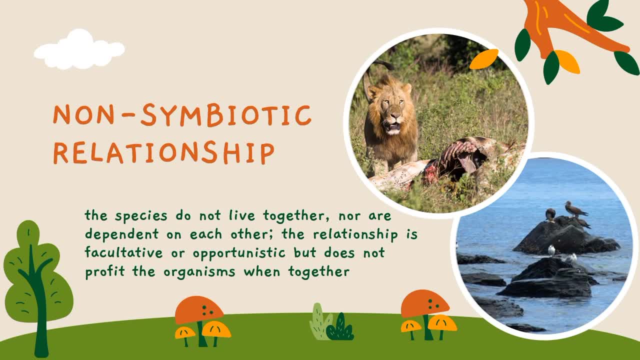 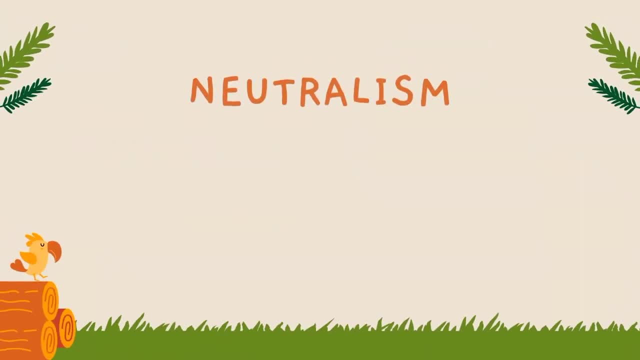 The relationship is opportunistic but does not profit the organism when together. One of the example of non-symbiotic is neutralism. When we say neutralism, it is the relationship between two species that do interact but do not affect each other. 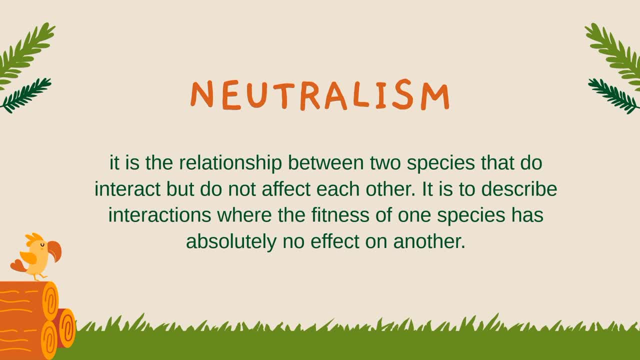 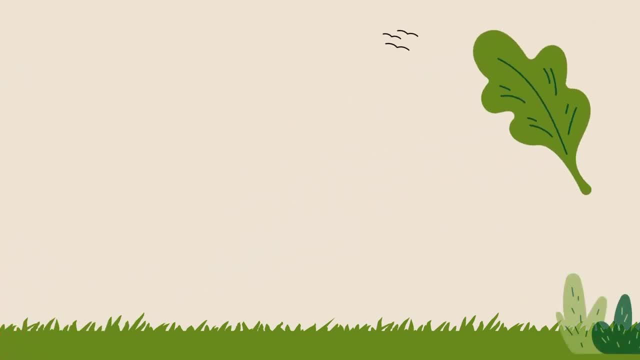 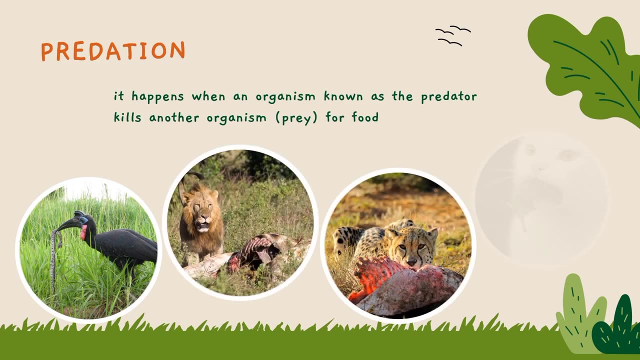 It is the interaction wherein the fitness of one species has absolutely no effect on another. Another example of non-symbiotic is predation. Predation is when one organism eats another organism for food. The organism that is eaten is called the prey. Another example of non-symbiotic is predation. 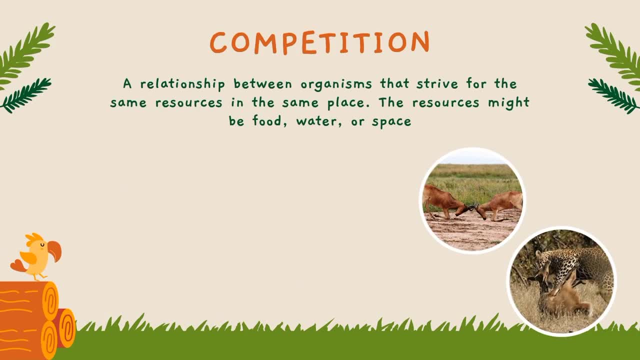 It is the relationship between organisms that strive for the same resources in the same place. It happens when organisms compete for resources such as food, space and territory. There are two different types of competition. It can be intraspecific or interspecific competition. 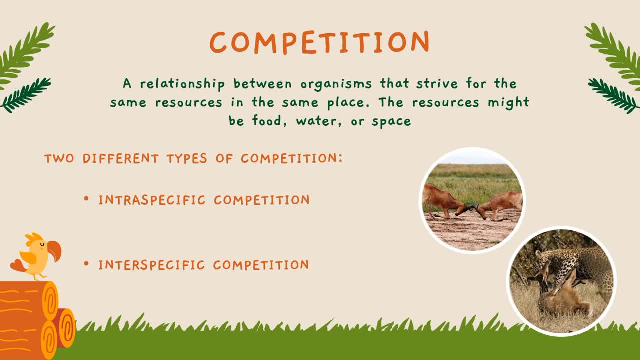 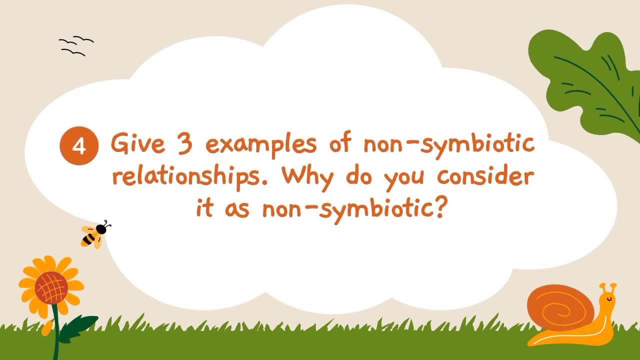 When we say intraspecific competition, it occurs between members of the same species. On the other hand, interspecific competition happens between the members of different species. Now give at least three examples of non-symbiotic relationship And tell us why do you consider it as non-symbiotic? 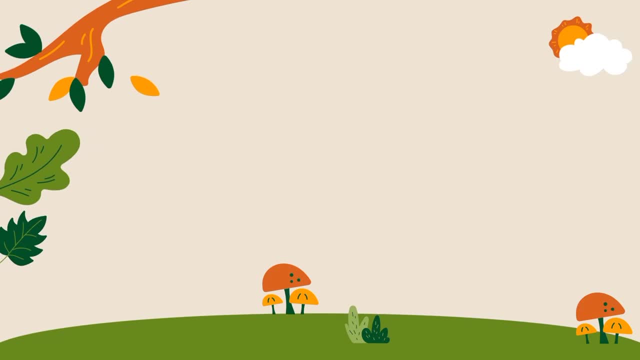 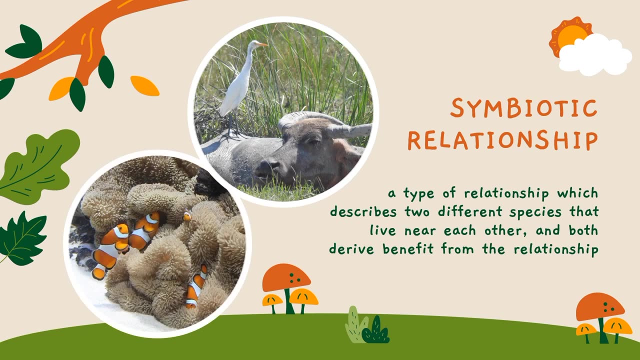 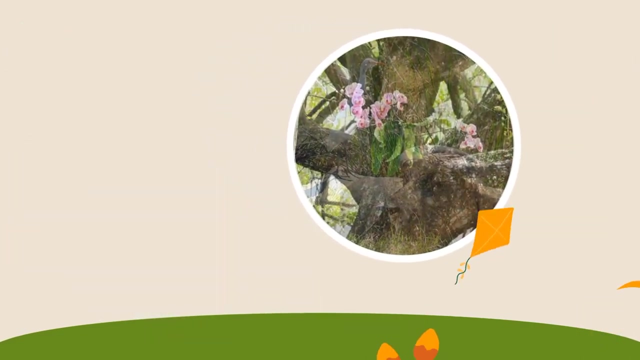 Now let us proceed with symbiotic relationship. When we say symbiotic relationship, it is a type of relationship which describes two different species that live near each other and both derive venison. What is the benefit from the relationship? One of the examples of symbiotic relationship is commensalism. 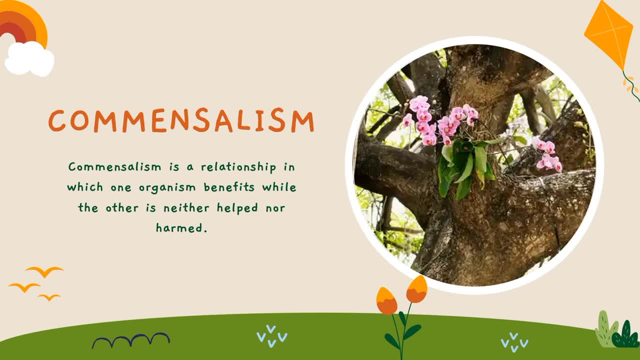 It is a relationship in which one organism benefits, while the other is neither health nor harm. For example, orchids that grow on the bark of a tree. The tree gains no benefit from the barnacle, but the orchids get shelter and space. Commensal is the one that benefits from the relationship. 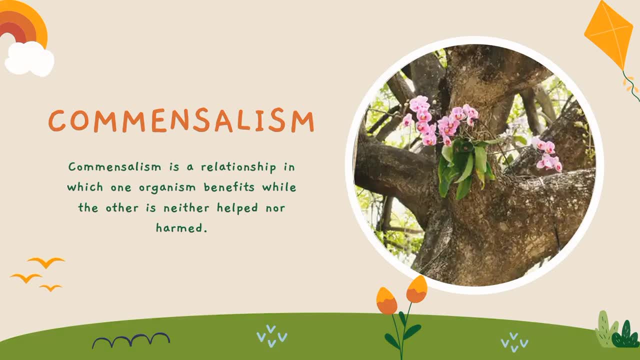 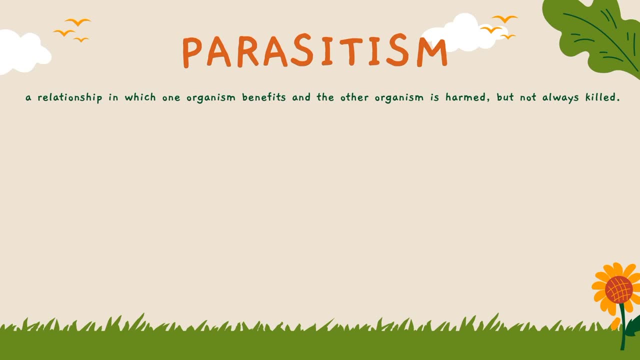 And in our example it is the orchid. It is the orchid. Another example of symbiotic relationship is parasitism. It is a relationship in which one organism benefits and the other organism is harmed, but not always killed. The organism that benefits is called the parasite, and the one that is harmed is the host. 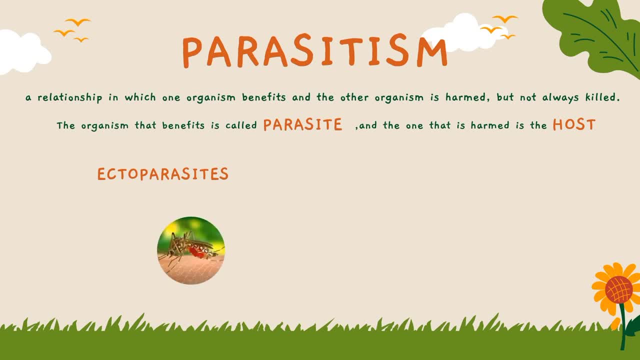 Parasites can be ectoparasites, such as mosquitoes, ticks, fleas and liches. Ectoparasites live on the surface of the host. Parasites can also be endoparasites, such as intestinal worms that lives inside the host. 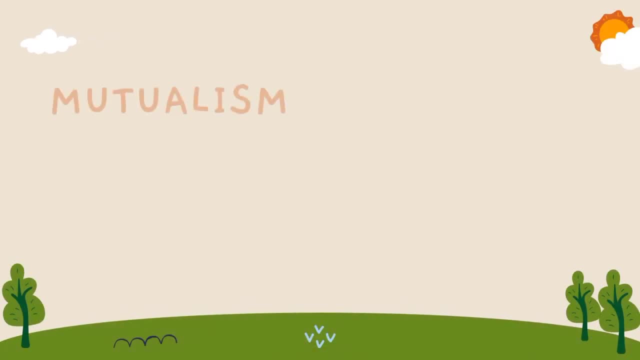 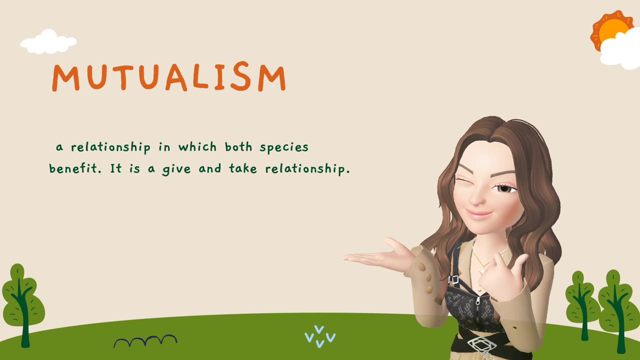 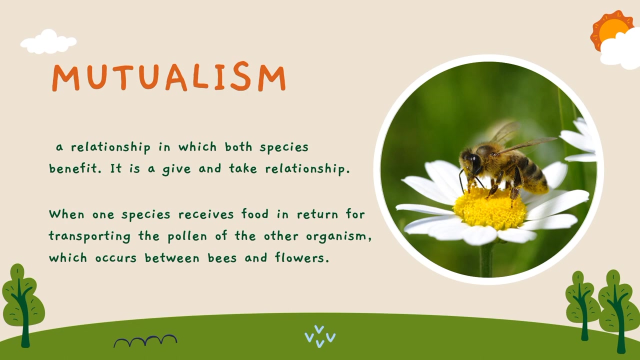 Another example of symbiotic relationship is mutualism. It is a relationship in which both species benefit, So it is a give and take relationship. For example, the relationship between bees and flowers: Bees receive food in return for transporting the pollen. Give at least three examples of symbiotic relationship. 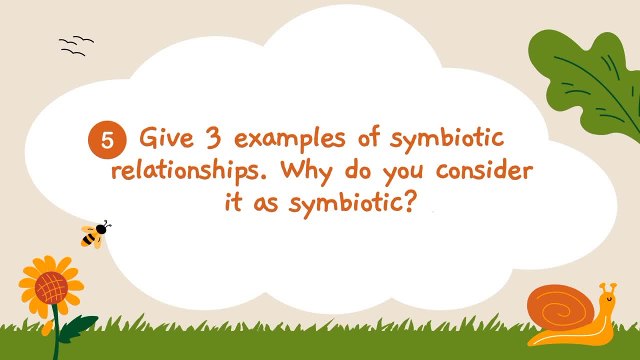 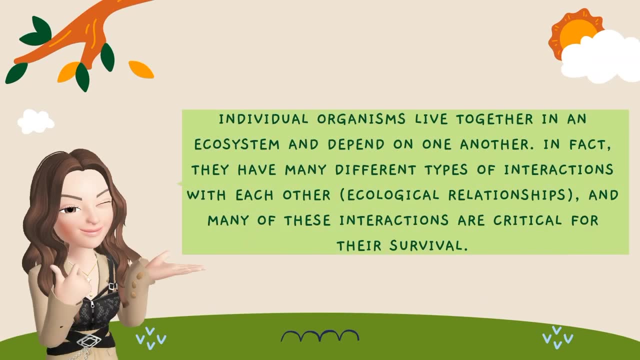 And tell us why do you consider it as symbiotic? Now, before we end this lesson, I would like you to remember that individual organisms live together in an ecosystem and depend on one another. In fact, they have many different types of interaction with each other, which is what we call the ecological relationship. 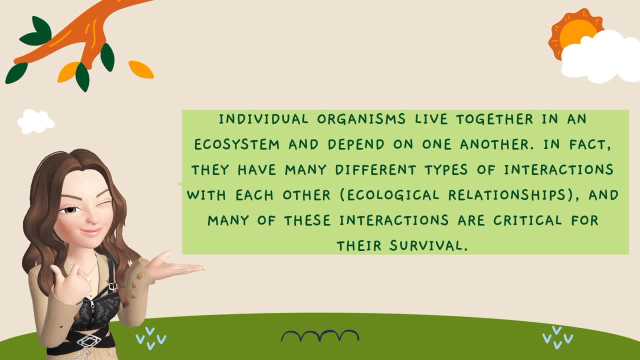 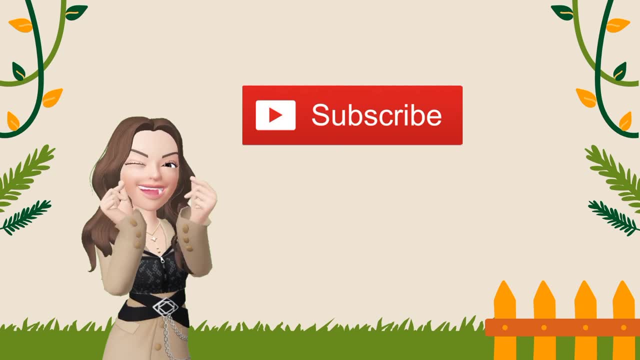 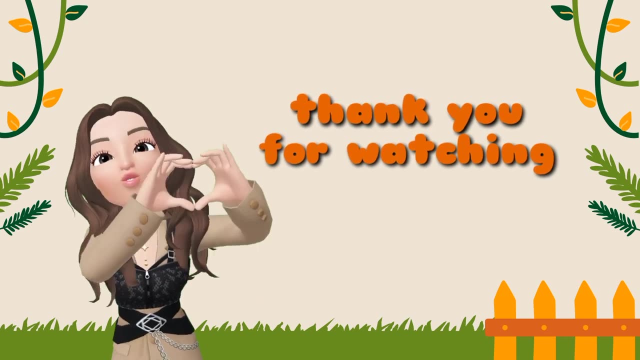 And many of these interactions are critical for their survival. So that's it. See you in our next video And if you are new to my channel, please don't forget to hit the subscribe button and hit the bell notification so that you will be notified for more videos like this. 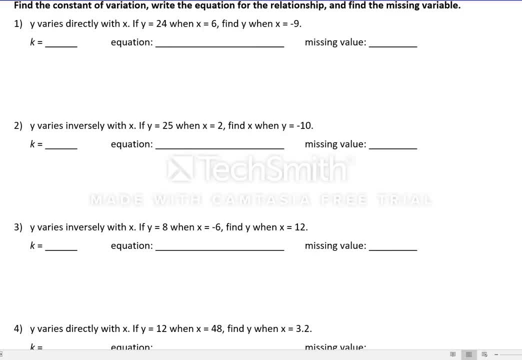 All right, all right, all right, We are looking at direct and inverse variation problems, equations, problems, finding the constant of variation, the missing values. We're going to get into some word problems. We'll get into some things where we can look at a graph and kind of identify what happens when x increases, and so on and so forth. 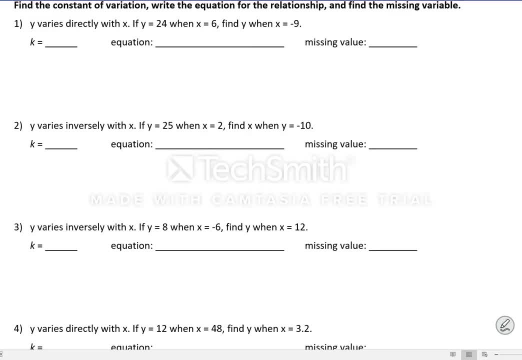 Okay. so before we do anything, we have to understand what's actually happening. So direct and inverse variation problems. So there's a specific equation to use for each type of variation. We have what we call direct variation. okay, and what direct variation actually is is? the equation is going to look like this: y equals kx. 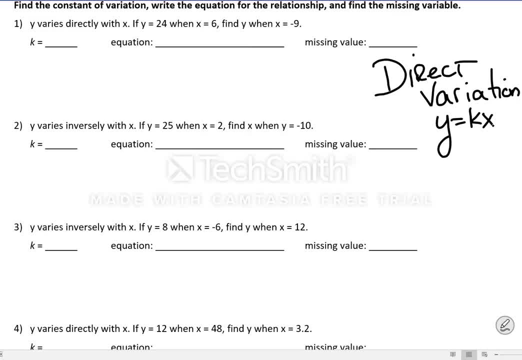 So y equals kx. it actually kind of looks like y equals mx plus b, just without the b. So this equation, if we were to graph it, it would always cross through the origin, okay, whether it be going up or down, depending upon the constant of variation. 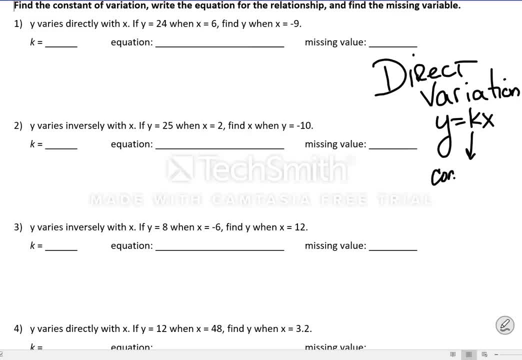 So k is what we call the constant of variation. You can think of it as your slope right, like the m value in your y equals mx plus b. That's basically what it is. Direct variation is equal to y equals kx. okay, so that's direct variation. 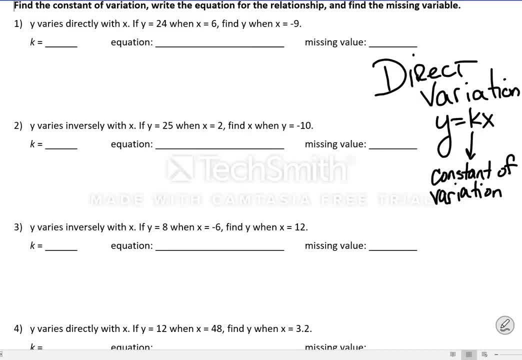 Now We have another one. It's called indirect variation, Indirect, Or it's called inverse Variation. Okay, they both mean the same thing. Indirect or inverse mean the same exact thing, And this particular equation is: y equals k over x.